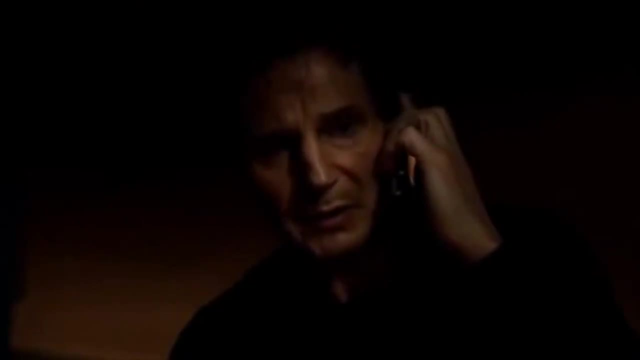 I don't know who you are, I don't know what you want, But I have a very particular lack of skills. I will never be able to find you, But what I do have is two dollars and a Casio wristwatch. You can have one of them. 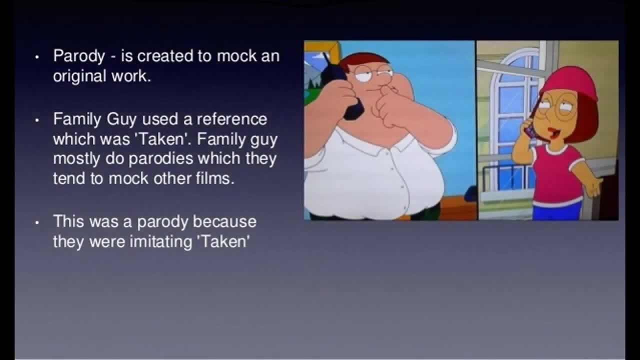 These guys are serious. To summarize, a parody is created to mock an original work And, of course, this episode was a parody, because it was clearly imitating the original works of Taken starring Liam Neeson. The important thing to remember about parodies is that there is no other meaning than to mock. 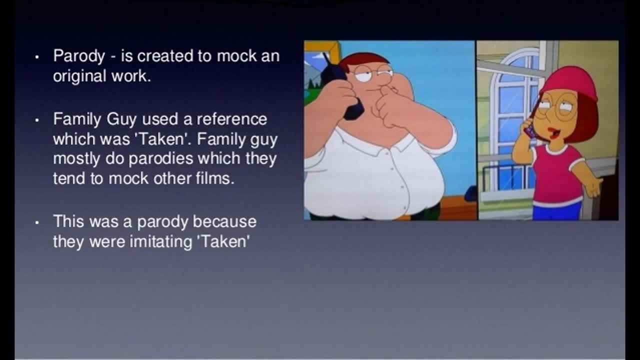 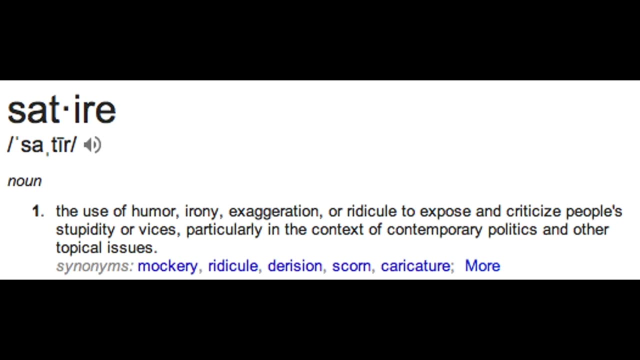 an original work. A parody is made for the sake of laughter and no further action is needed from the audience. This is a good time to go over what a satire is, since satires have a different purpose. A satire is the use of humor, irony, exaggeration or ridicule to expose and criticize. 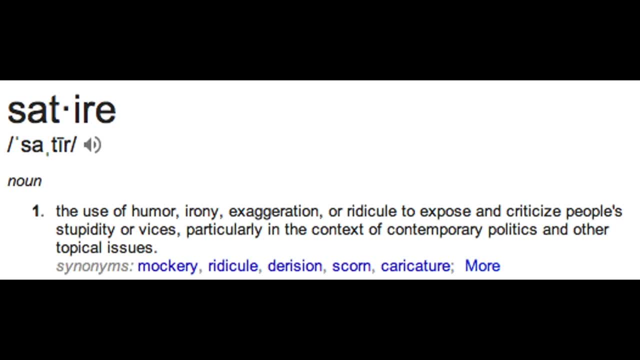 people's stupidity or vices, particularly in the context of contemporary politics and other topical issues. I know that is a lengthy definition, but understanding a satire is really quite easy. Let's use the other show that I mentioned at the beginning of the video to make the 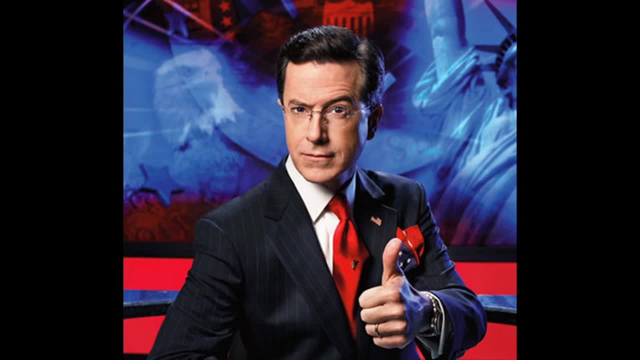 definition of a satire a lot simpler. Colbert Report is an American late-night talk and news satire television program hosted by Stephen Colbert. It is a show that mainly talks about current events, and Stephen Colbert acts as a news anchor who is overly patriotic to purposely make humorous comments on the issues that 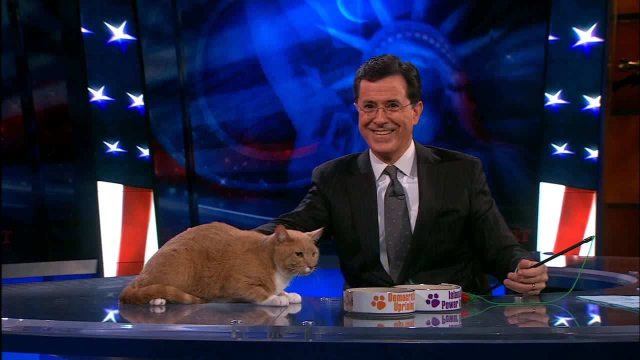 he is addressing. Sarcasm is a huge factor in his show, since most of the time he is saying one thing, but he means the exact opposite. It would be a lot simpler to actually see Colbert in action, so let's take a look at a quick clip of one of Colbert's stories. 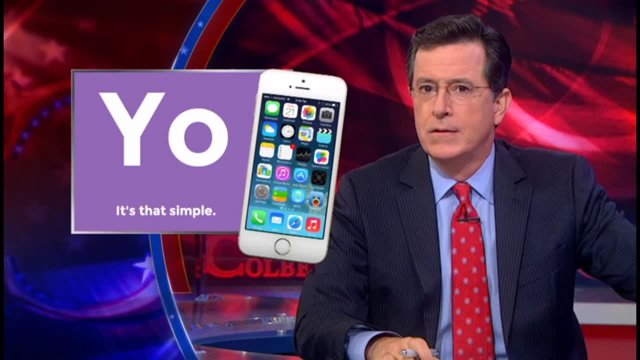 Let me give some background info so that you aren't completely lost In the clip that we are about to see. Colbert is talking about a new app that is called Yo. Basically, it's an app that allows people to message each other with only the word Yo. 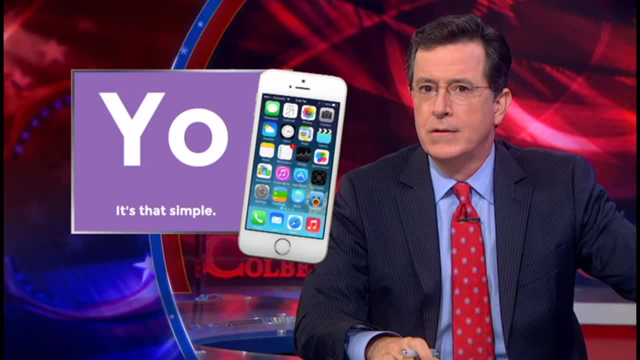 The app's description, as seen in this picture, is: Yo. it's that simple. The clip we are going to watch shows Colbert talking about a new app that is called Yo. Basically, it's an app that allows people to message each other with only the word Yo. 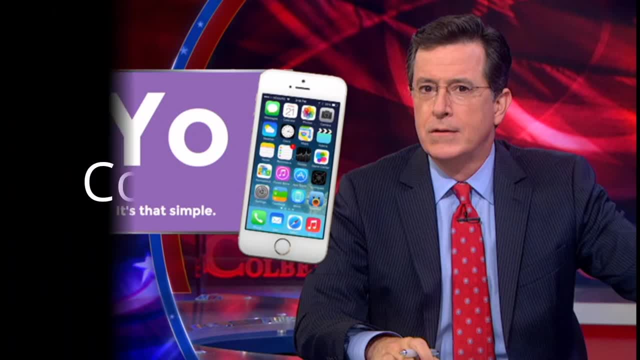 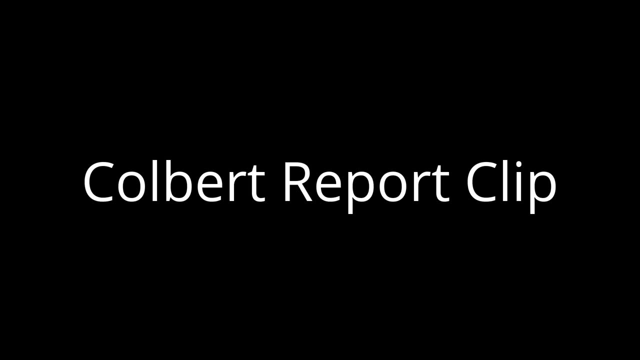 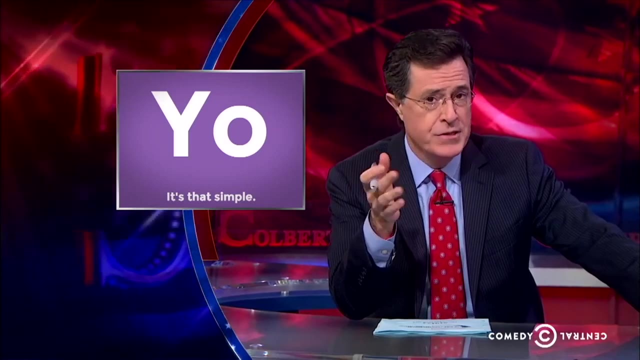 The clip we are going to watch shows Colbert's reaction to the app. Afterwards we will talk about what he is literally saying versus what he actually means. When I first learned about an app that boils down all your communication into two letters, I expressed myself in one